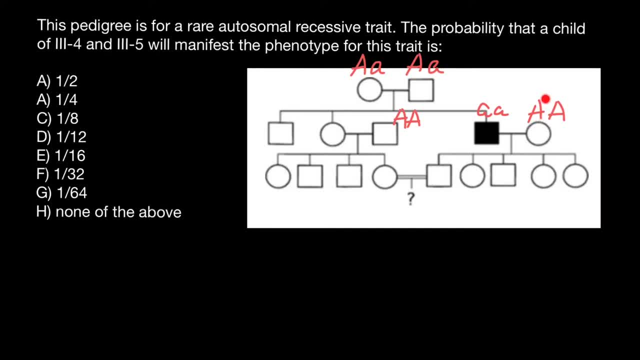 children of this couple. from mother side they only can get dominant allele and from the father side they only can get recessive allele. so we know that for sure this person here is obligate heterozygous and the probability is going to be 100 or one. so again, all children of this couple are going to be heterozygous. 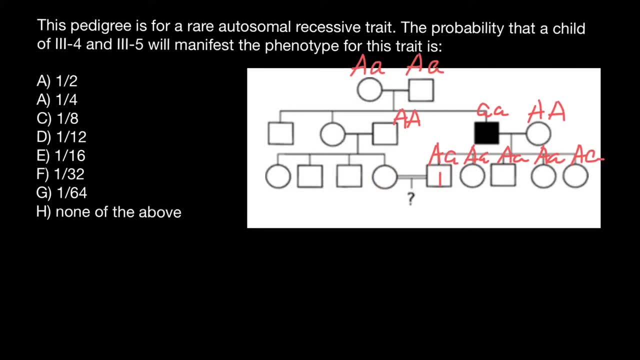 now let's find probability for this person to be heterozygous. and we know that father is homozygous, normal, dominant. and what about mother? we know that her phenotype is normal, but what is her probability to be heterozygous? take a look: we know that her parents are heterozygous and we can build simple planet square and here what we 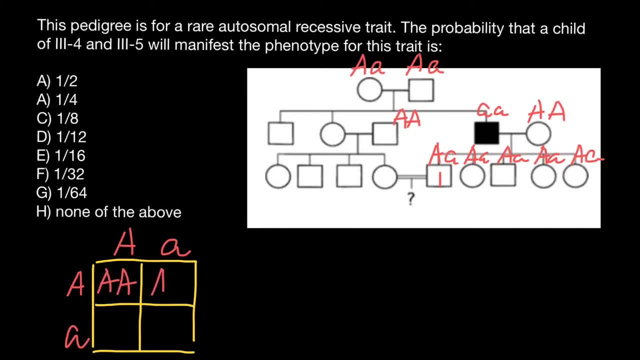 are going to see capital a capital, a capital a small a capital a small a and small a small a. we know that this female is not homozygous, recessive or she would be affected, so we can exclude this variant. now we have to choose. what is the probability of this female to be heterozygous? or to be a carer, sorry in English. for some reason I am not sure that this is correct or not. The probability of this female to be heterozygous is 100.. Her probability is going to be 50.. So let's see the results. 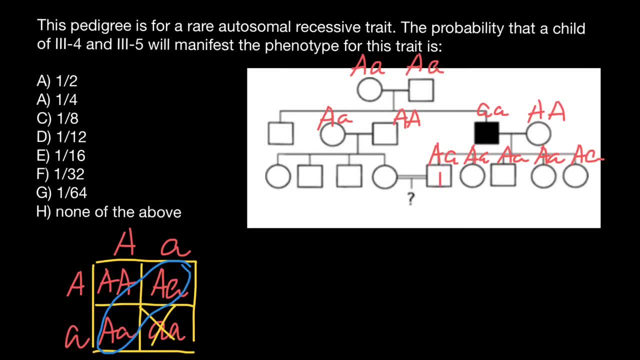 going to be 2, not out of 4, but 2 out of 3, because again, we excluded this variant. so this is going to be your probability: 2 thoughts to be heterozygous. now let's find probability that your daughter is going to be heterozygous and 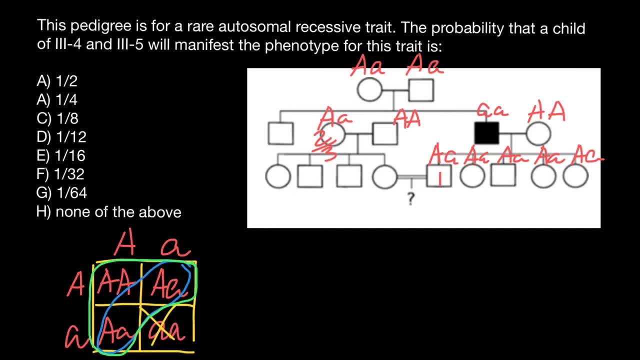 probability that your daughter is going to get dominant alleles from the father side is going to be 100%, so we know that one allele is dominant. what is the probability for a daughter of this couple to get recessive allele from the mother side? take a look: 50% that this is going to be. 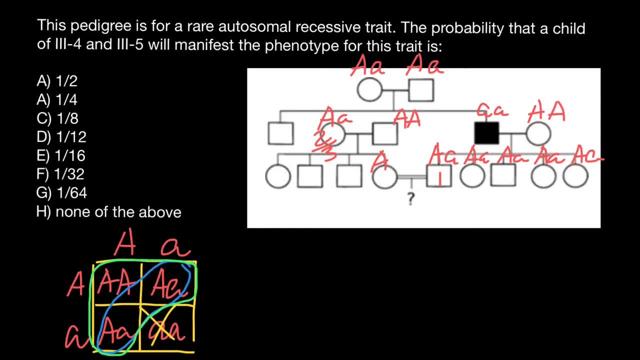 dominant allele and 50% that she is going to get recessive allele. so we can say that probability is going to be dominant allele. so let's find probability that your daughter probability is going to be one half that this female is going to get this recessive allele. 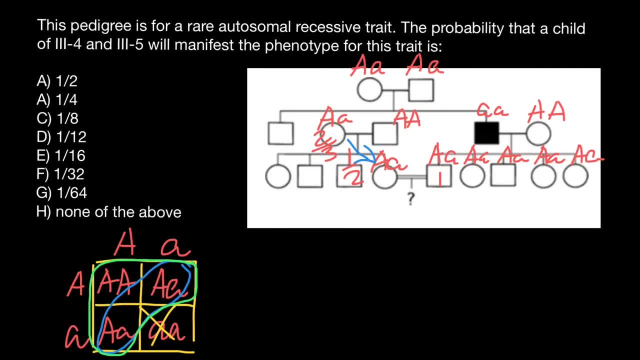 from her mother. now we can do our final calculations. so probability for this female to be heterozygous is going to be two thirds times one half, so it's going to be two, 36, and we can reduce these numbers and we are going to get one third. this is going to be: 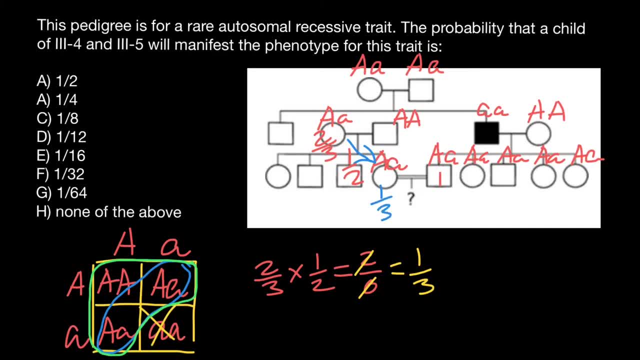 probability for this female to be heterozygous, and we know that this male here, 100%, is heterozygous. we also can say that one is the same as one over one. if we know that two parents are heterozygous, we also can find probability for this couple. 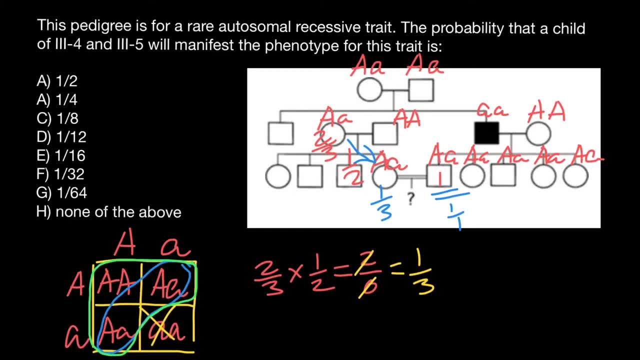 to be heterozygous. we can find probability for this couple to be heterozygous, have homozygous recessive child and, as you see, the probability is going to be one quarter, one out of four. and now we have also multiply, if you like, we can multiply by one over one. this is 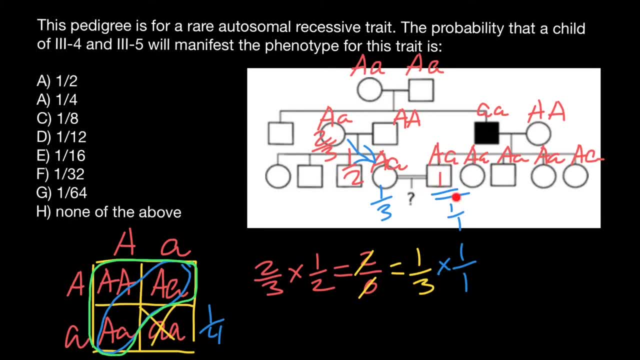 probability for this male to be heterozygous. it doesn't affect our calculation, so we can just exclude it. and we also have to multiply by one quarter. by one quarter that if this couple are heterozygous they are going to have homozygous recessive child, our final answer is going to be: 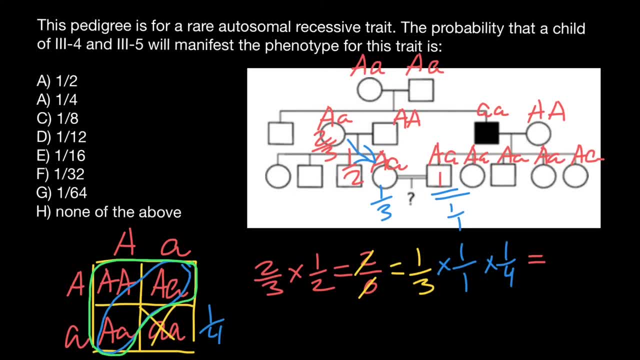 one third multiplied by one quarter, one twelfth, and this is going to be our final answer: probability for this couple to have affected child of unspecified sex would be one twelfth, and this is all for today. thank you for attention. please subscribe for my new videos that i post almost every day. 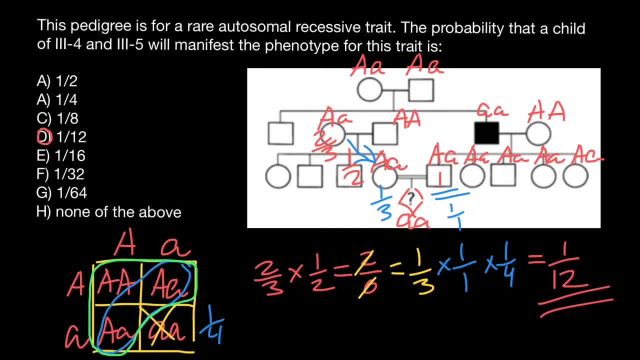 and see you in the next video. goodbye you.